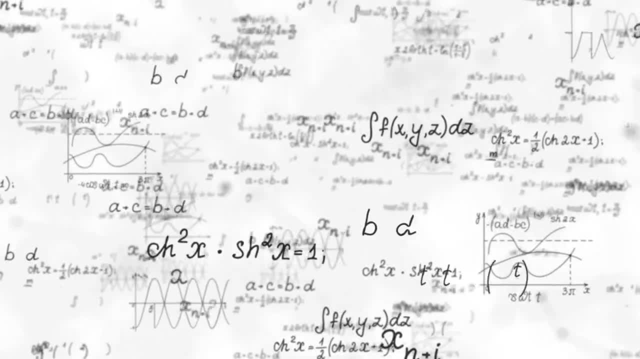 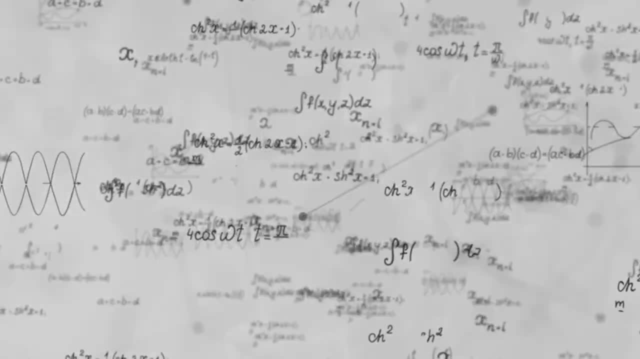 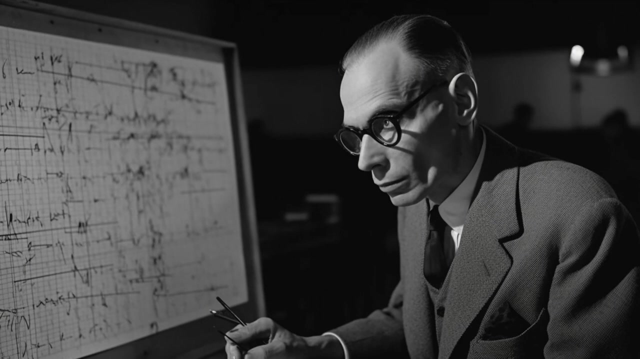 the confines of a given mathematical system. Challenging the dream of complete formalization, The early 20th century saw an ambitious project by mathematicians and logicians like Bertrand Russell and Alfred North Whitehead. They hoped to formalize all mathematics into a set of axioms, from which all mathematical 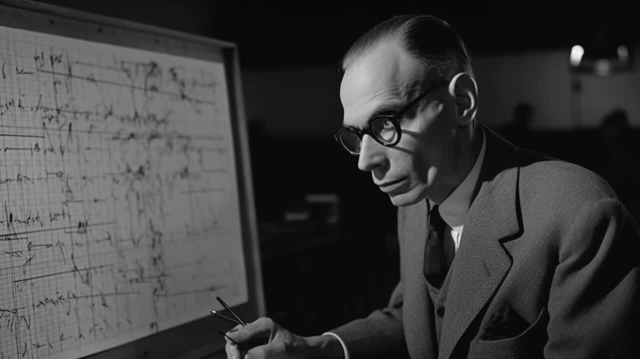 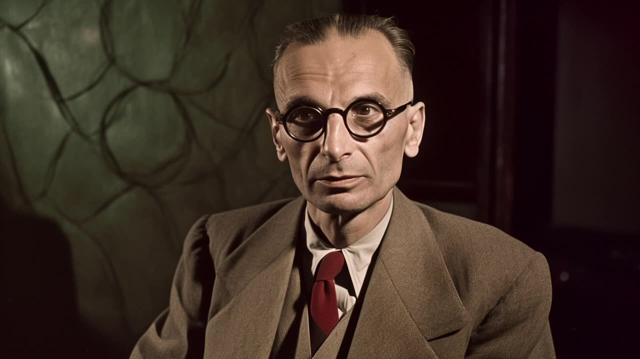 truths could be derived. Gödel's theorems were a major blow to this dream, showing that no single system could encapsulate all mathematical truths. Gödel's theorems draw a clear line between what is true and what can be proven. 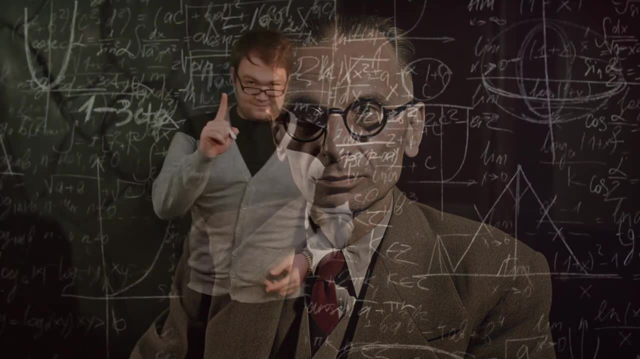 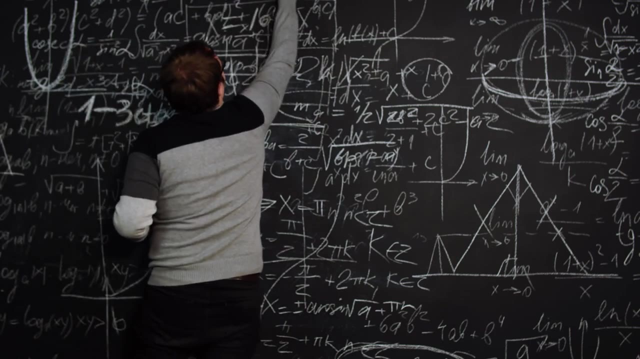 Just because something cannot be proven within a system doesn't mean that it's not true. This distinction has deep philosophical implications touching upon the nature of truth itself. Limitations of a system where Sure Law and Dare are tatners are not sound topretation for manuscript flows. 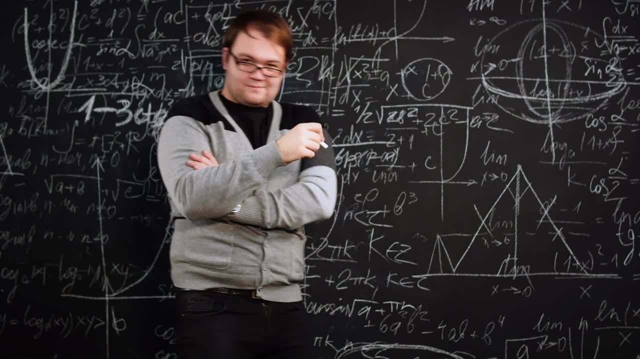 Limitations of a system where Sure Law and Dare are not sound. topretation for manuscript streams betterender is false in the defense of what is true, either plane or polytheistic of rational thought, If even mathematics often viewed as the most rigorous and logical discipline. 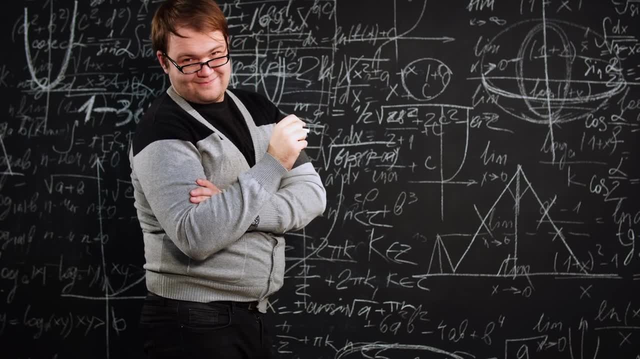 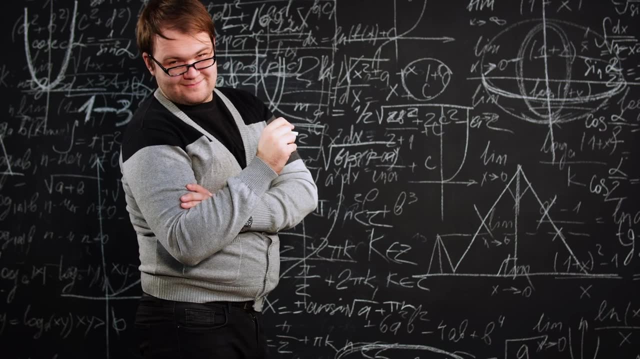 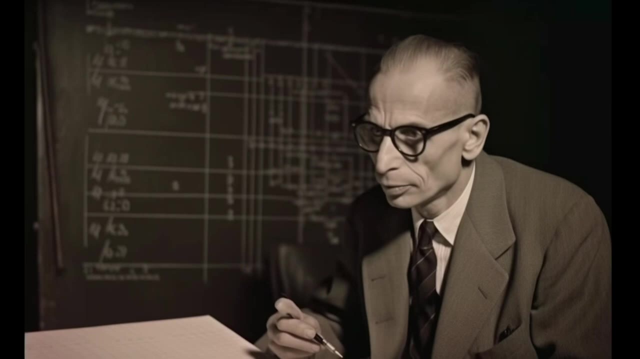 has its limits. what does this say about human reason in general? The theory implies that there's a boundary to what can be achieved through structured logical processes, Metamathematics and levels of understanding. Gödel's work gave rise to a study of metamathematics. 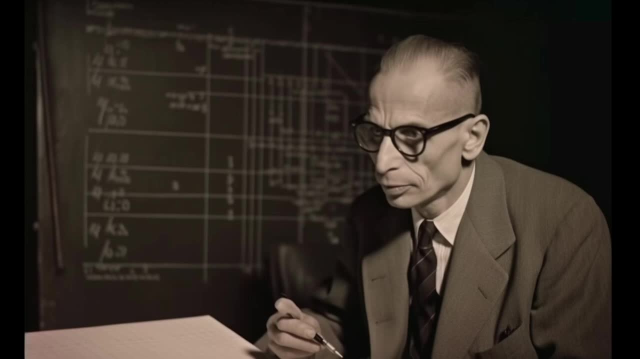 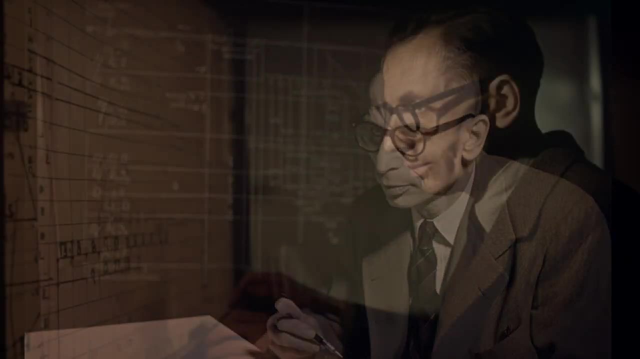 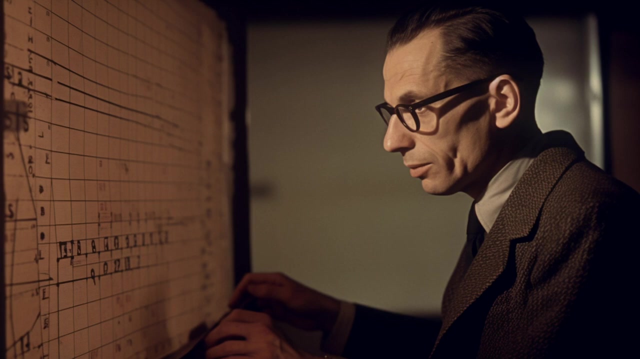 the investigation of the foundations and properties of mathematical systems. It suggests that to understand certain truths of a system one has to step outside of that system. This has parallels in philosophical discussions about levels of consciousness and understanding: The human mind versus machines. A popular interpretation of Gödel's work is his 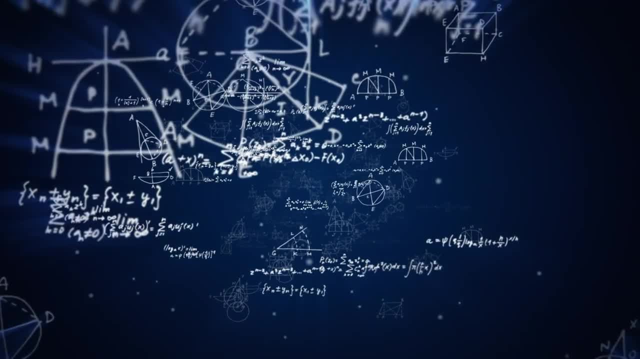 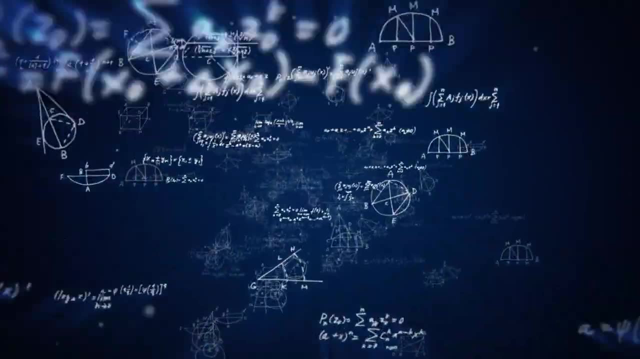 argument against mechanism which claims that human minds are in essence machines. Gödel's theorems suggest that there are things the human mind can understand, like the theorems themselves, that cannot be derived from any formal system. If the human mind were just. 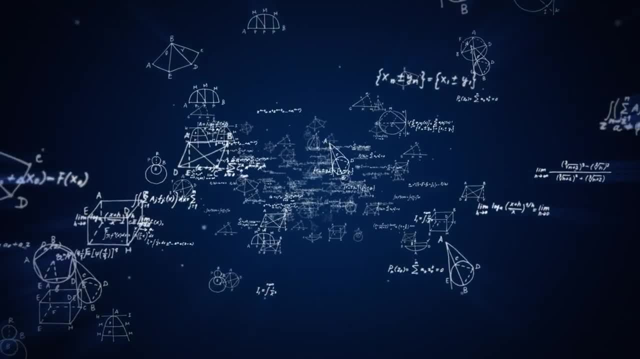 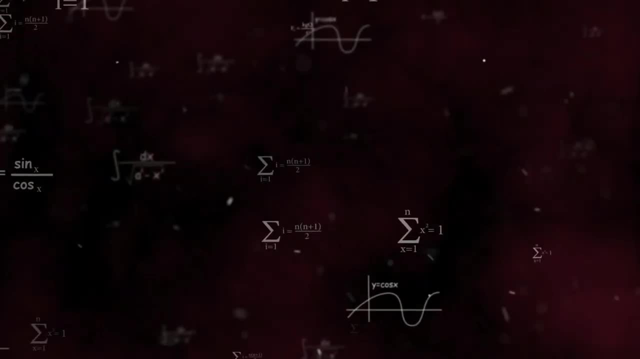 a type of machine, it wouldn't be able to understand these things, leading to the idea that perhaps consciousness or understanding is non-mechanical or non-computable in nature. Gödel's incompleteness: theorems might be based in the realm of mathematical logic.